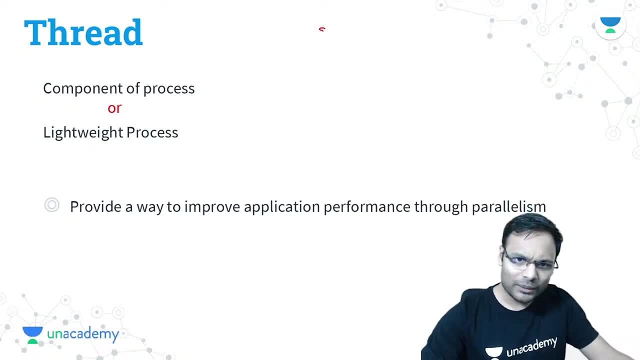 full-fledged facility. So whenever a student was coming, that fellow was building a new house for that and giving it for the rent. So that fellow, what that particular fellow was doing, The fellow was building a particular flat for that student, A particular flat for that student. In that flat the student 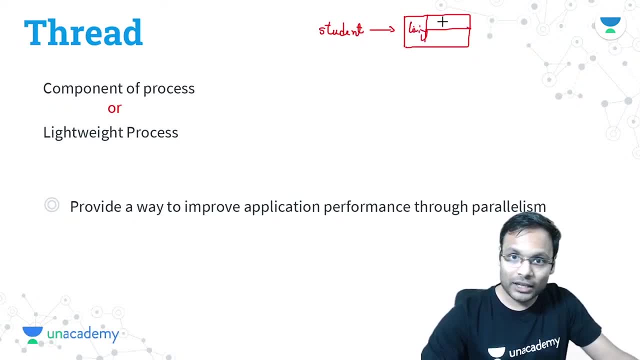 had a particular living room, a particular kitchen and bedroom. Then another student came. second student number came Thus for second student also. that business person has built the same kind of flat in which living room was there, then bedroom was there. 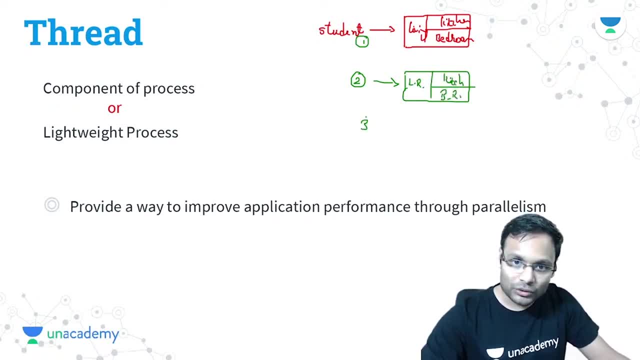 And kitchen was there. Then for number 3 also, number 4 also, number 5, also number 6 also, The businessman understood that every student coming for college, or maybe coming for coaching or something, They are spending their maximum time in bedroom for study and all. 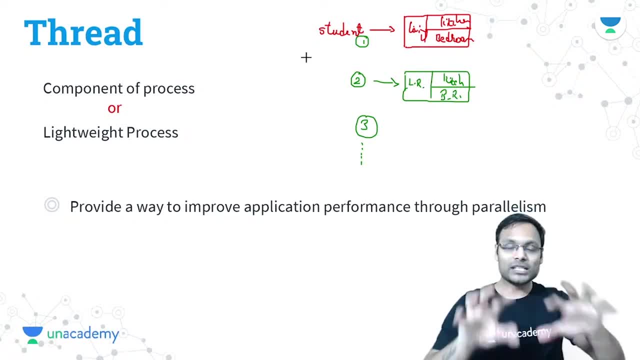 They are just maximum time. they are spending time in bedroom only studying, studying, studying or sleeping, studying, sleeping. That's it The kitchen they are using very less time. Living room also very less time, But it's my wastage. 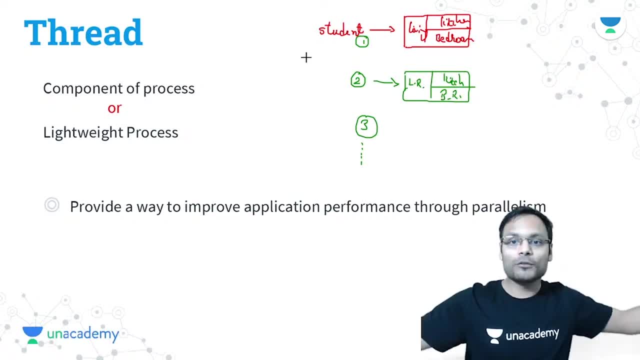 This is my waste? Why? Just because that fellow has given a lot of space Kitchen and it's so many accessories in the kitchen, A full-fledged kitchen. that fellow is giving and providing to the student, But students are not utilizing it. 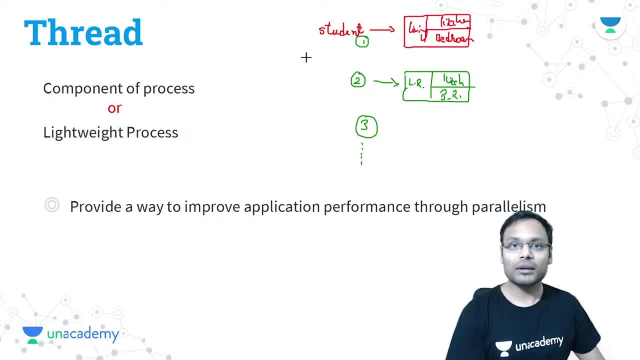 Students are not utilizing it, But it's a waste time, Right? Why? Just because that fellow is giving living room to each and every student separate, separate. Giving kitchen to each- Each and every student separate, separate. Bedroom- each and every student, separate, separate. 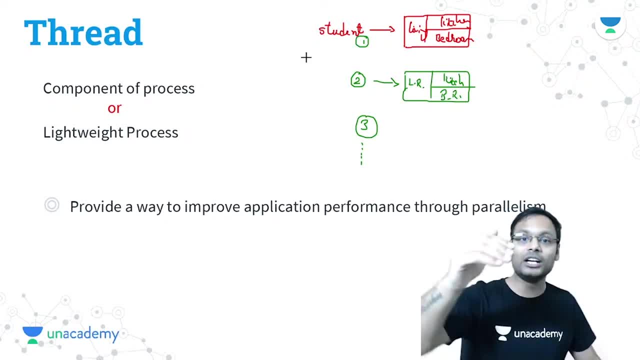 And such kind of 100 students are coming. He is building 100 flats in that particular area. It's a wastage of space. It is a wastage of space, wastage of money, and the return of the money is also not there. 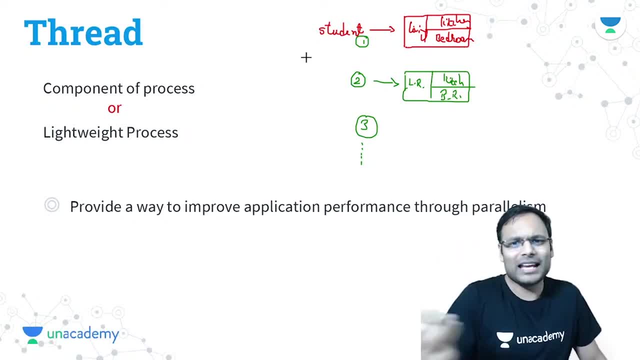 It's a mistake, The fellow will think like that. So what other business person? the competitor thought that Competitor has started another business of same type. Now competitor is doing what The competitor is saying, that whenever a student comes, that fellow has built one common living room and a common kitchen. 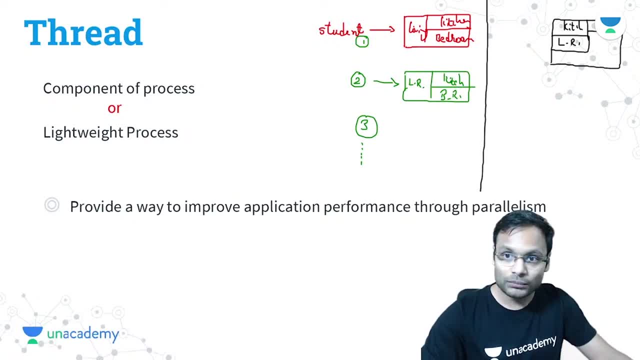 After that, for each student, that fellow was building a bedroom. Only that fellow was building the bedrooms for each and every student. What happened in that case? What happened? What happened in that case? What happened? Kitchen got shared between multiple bedrooms. 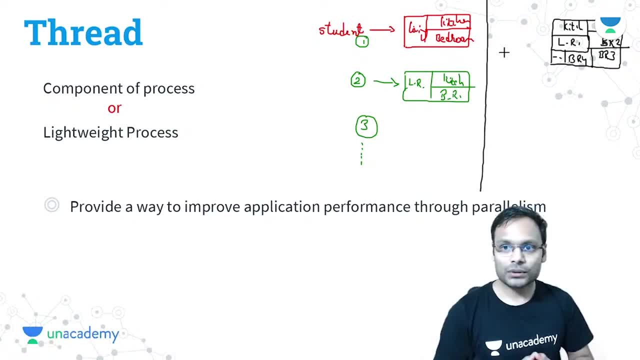 Living room shared between multiple bedrooms. In that particular case, second businessman is earning more money, saved a lot of space, lot of money also, and return of the money is also good. You know why? Just because every time a new student comes, I will not have to replicate entire flat. 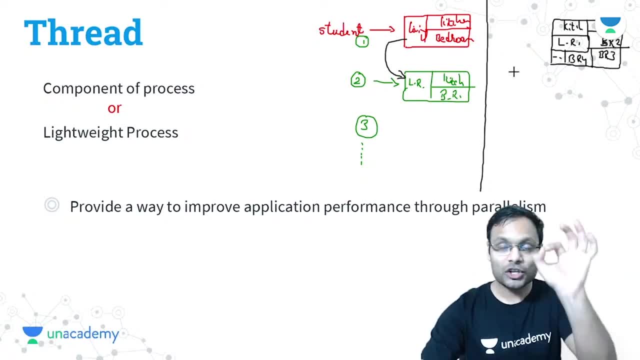 I had to replicate only one thing, which is required separate, separate, for each and every student: a bedroom for sleeping and studying. Understood Here. in this particular case, what happened? The second businessman was earning better, And this is what the basic concept of thread. 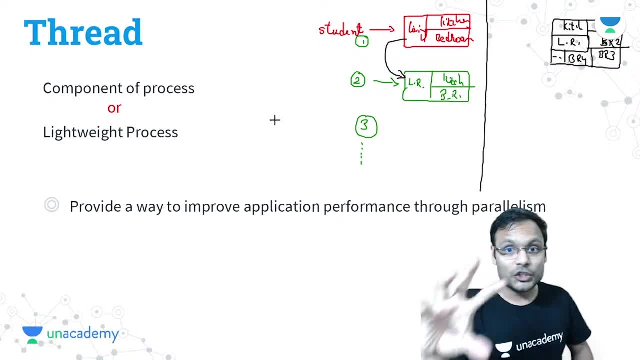 Basic concept of thread. Now let me just put this example into your real operating system. example: If suppose there is a process- student is a process, Let's say: okay, so there is a process. that particular process is doing some work. 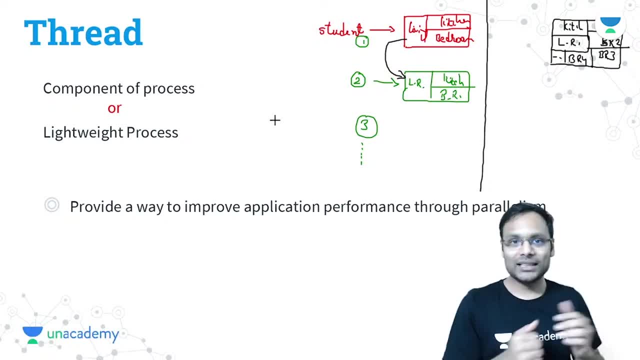 Suppose my requirement is like this: that I will have to perform the same operation, same particular process. execution I want, But I need to A very simple one. Then two instances of that. two instances. Why two instances? Just because for two different data I need to perform the same operation. 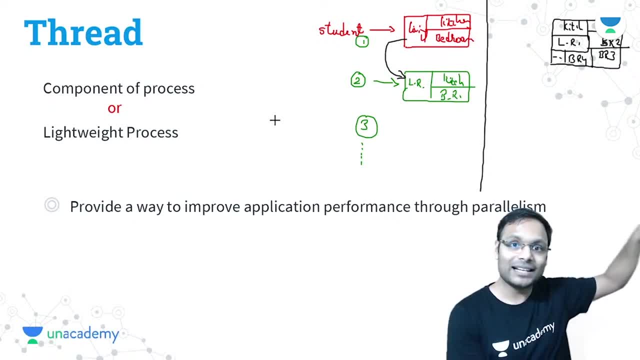 It's like a web request. We'll you said a way of request. There is a process- listener process- at the end of Google's server. I've send it, But that's not the only request. are there multiple requests? So that listener? 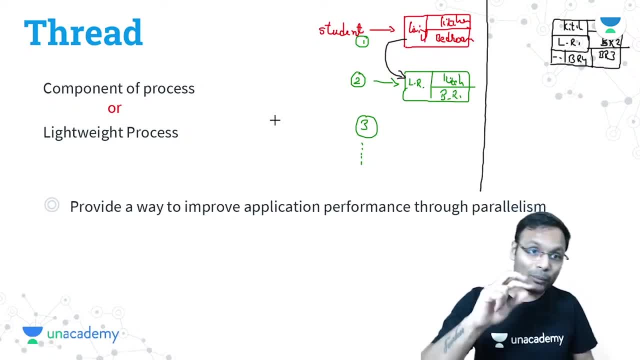 For as many as requests are coming. But the problem here is, if you are replicating the processes, it will be a very tedious task. Same operation, same code, Only few things are changed in two process instances, But you are replicating entire process.